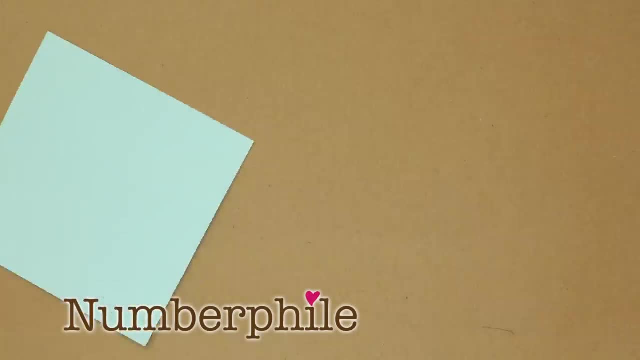 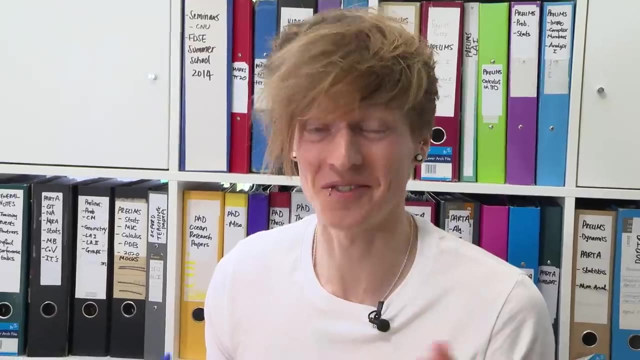 Today we're going to look at my favourite puzzle. It's involving squares, rectangles. I've actually used this a few times in the Oxford University Admissions interview questions, so it's got some heritage behind it, a bit of prestige behind this question. I won't be using it anymore because I'm 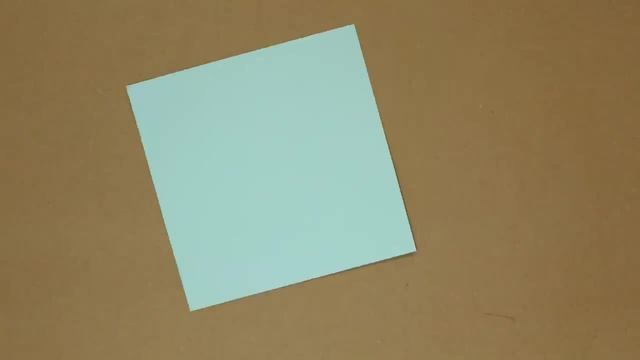 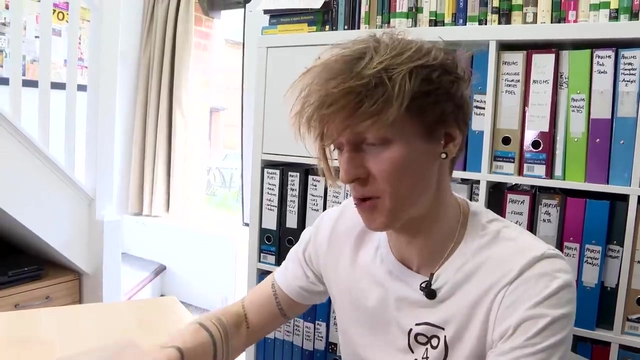 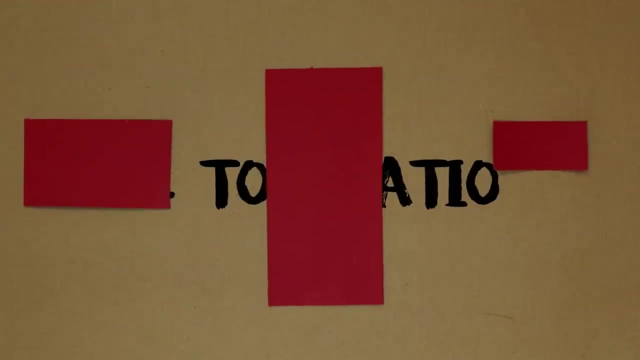 going to tell you all how it's done. We're going to start with a square like so, and this can be any size square, it doesn't really matter- and what we want to do is fill the square with rectangles. Now, the rectangles can be of any size as well, but they have a rule that they have to be in the ratio. 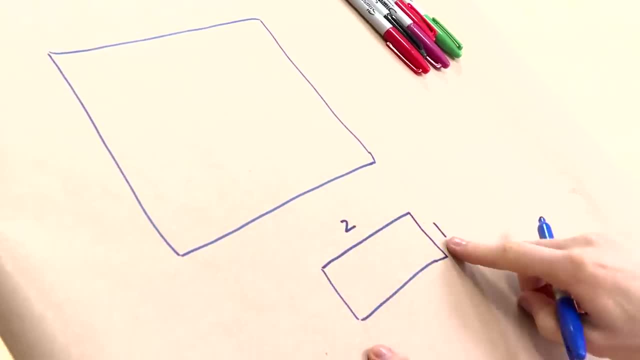 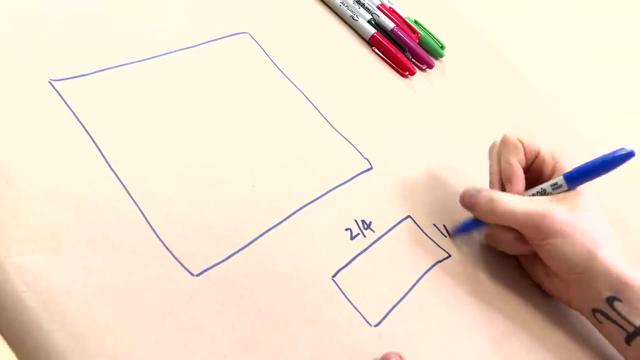 two to one. So this doesn't mean this is length two and this is length one. this could be length. let's say this was two quarters and then, oh, I should have picked a better number and this one needs to be one quarter So we could have smaller ones and really tiny ones. 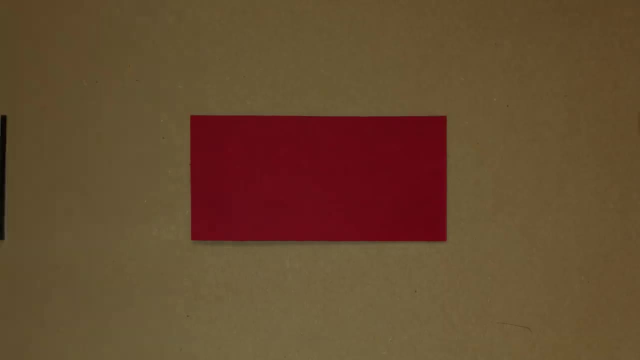 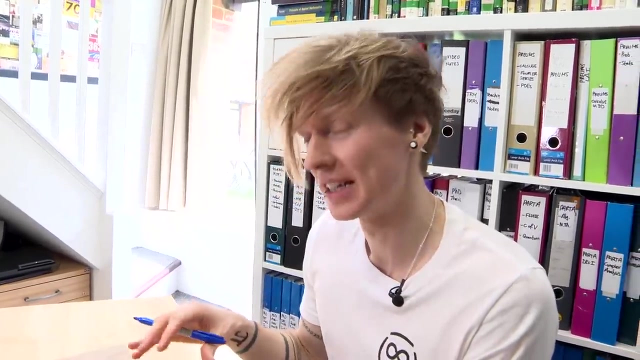 it doesn't matter the size of the rectangle, they just have to be in this ratio: Long side is twice the length of the short side, and what we want to do is fill the square with these rectangles, and we're interested in for what numbers of rectangles. 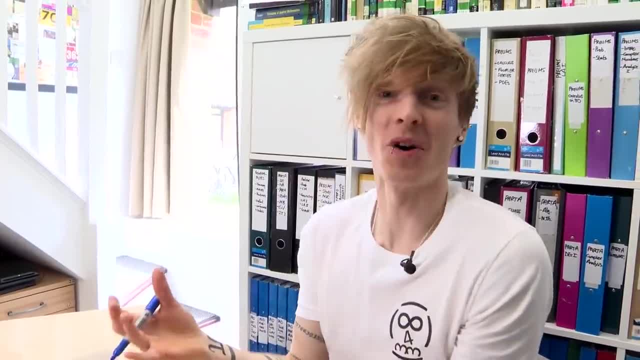 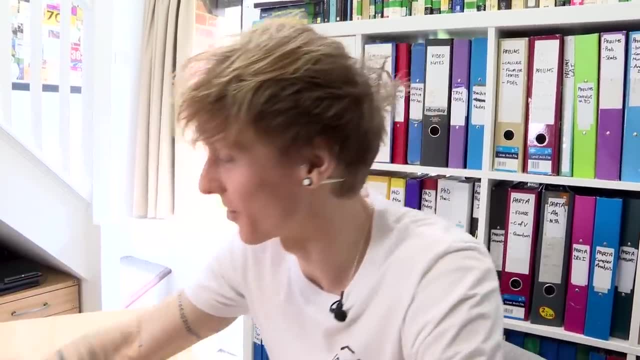 is it possible to fill the square So clearly for one? it isn't, because a rectangle, in this ratio two to one, is not a square, so you can't just fill it with one. So we can say, for n equals one, that's a big no, but then for n equals two, it's going to work because I can just do that. 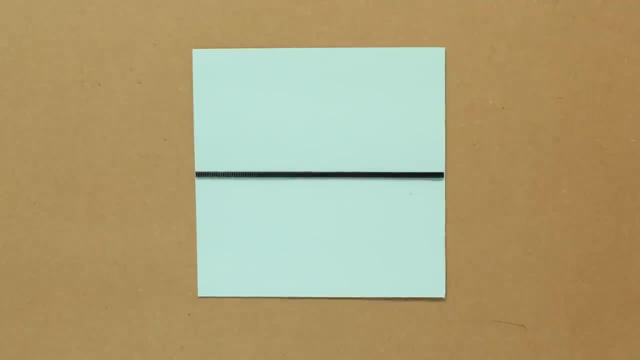 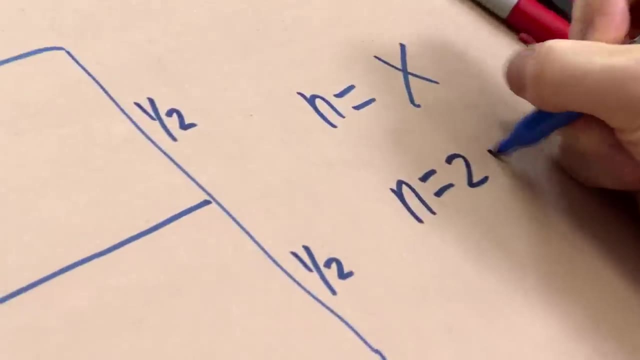 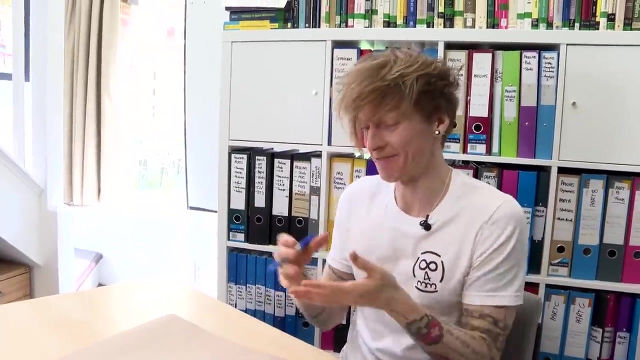 If we say the square is one by one, then both of these rectangles are one by a half, twice in the ratio, and we can fill it with two. So n equals two is a tick, and that was n equals one was the cross, And we want to know for what other values can we do this? Is it possible for any other? 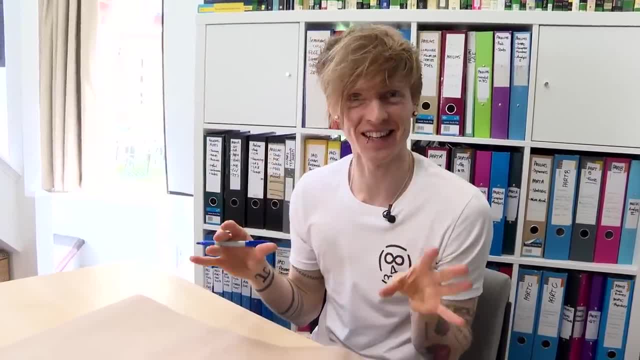 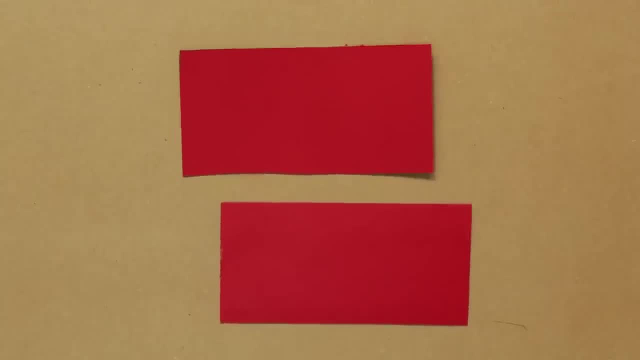 values. Can we do it for all of them? That's the question. can we figure this out So you can use duplicates? obviously, Yes, we can use the. so here we've got two of the same size. I could have it. 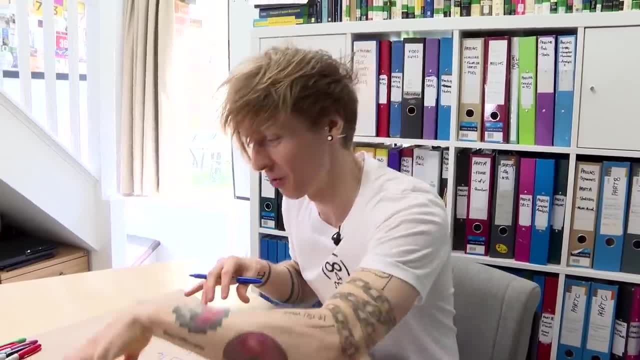 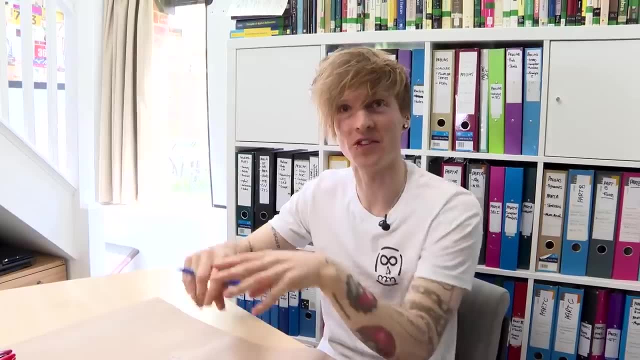 doesn't have to all be the same size, so that's important. We could have one big one and, I don't know, six small ones or something, Or maybe like four different size rectangles. There's no limit in the size of the specific rectangles or the numbers of each one, just we're interested in the total number of rectangles that. 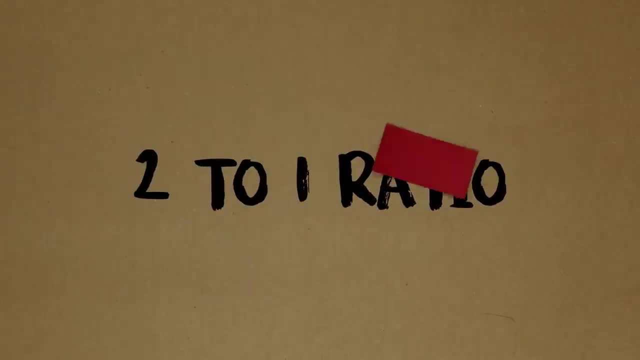 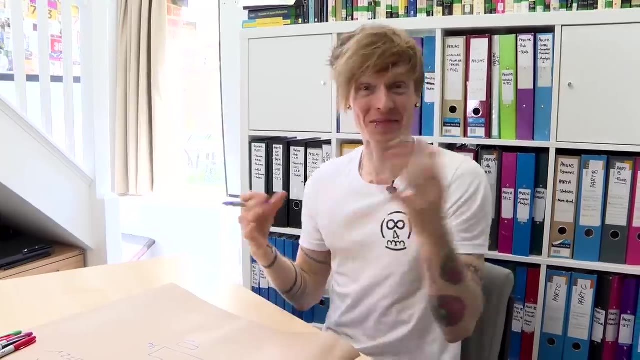 fill the square as long as they're in this ratio. So is the puzzle question: for which numbers can we do it? Or is the question: can you do it for all numbers? Or, like I always thought about, I always present it as: for which numbers can we do it? But within that we're kind of saying: 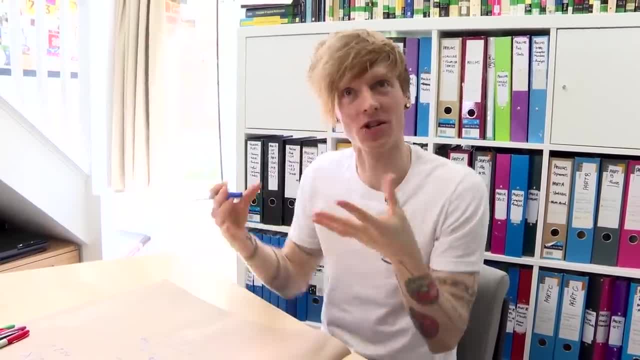 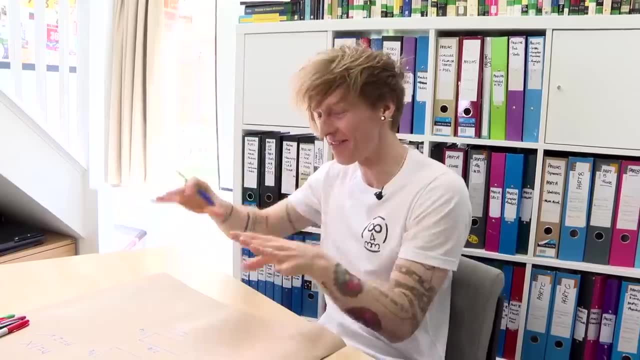 can we do it for all numbers? Are there some numbers other than one where it doesn't work? But we're going to, hopefully. we're going to try and consider all possible values. that's the goal: We're going to actually try and consider every single number. So the way I would approach, 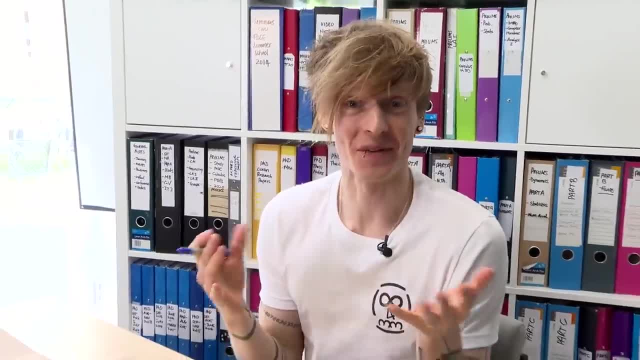 a problem like this is: well, there's two options, the way I see it. So we've shown so far it's not going to work for one, because then it would be a square, and we've shown that we can do it for two. 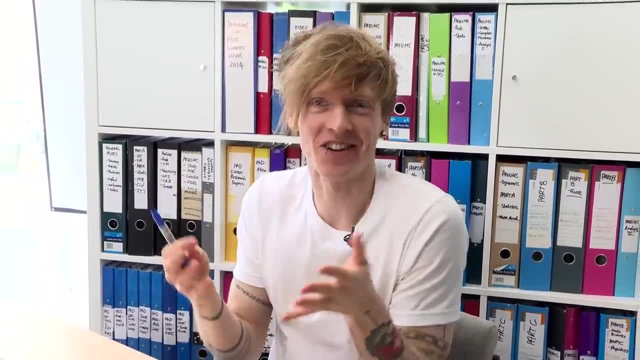 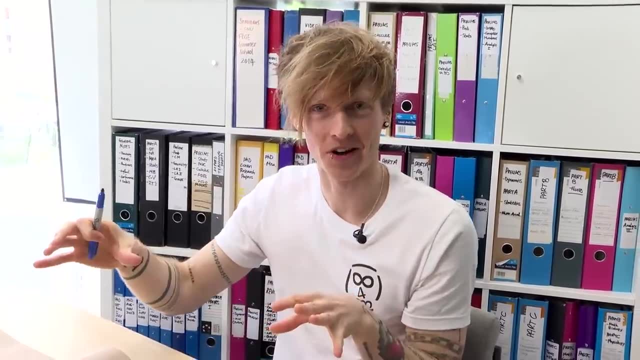 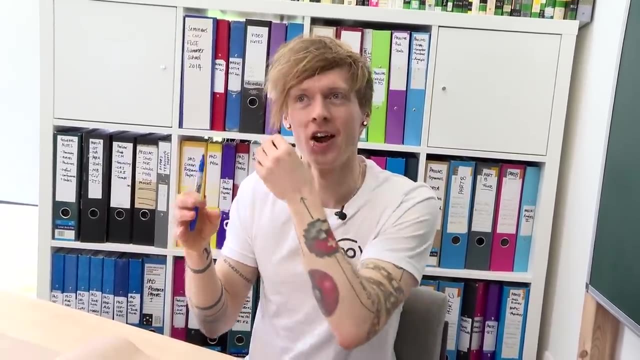 So you could continue in this way and say: well, let's try and do it for three, let's try and do it for four. But the problem is, if you hit a number where it doesn't work, you've got to show it doesn't work. You've got to like: try everything, like. you have to exhaust all possible. 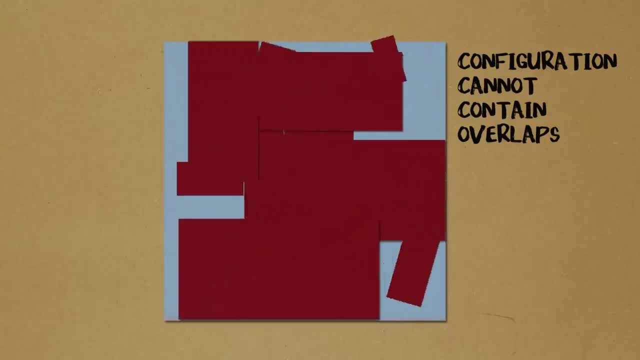 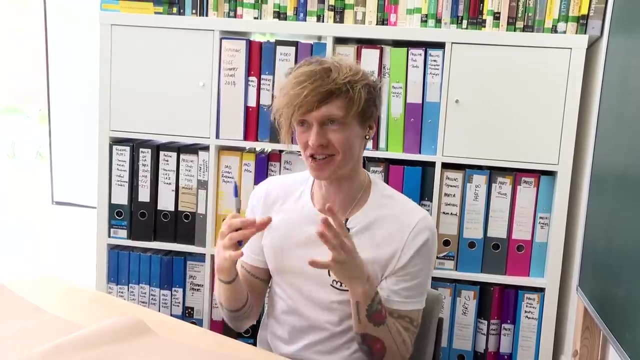 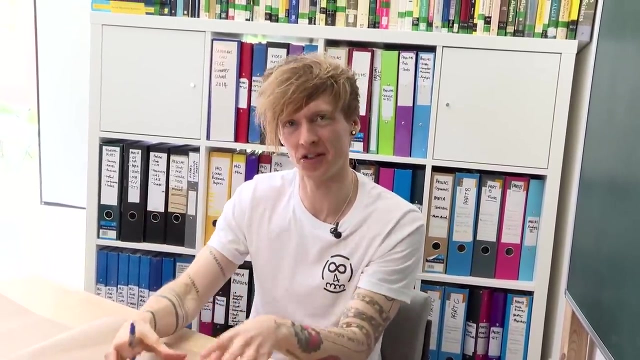 ways of arranging rectangles, and it's really difficult to exhaust every single possible thing that you can do in such an open problem like this. So my suggestion would be to think: well, can I find something else that works that isn't two, Let's try and get like another handle on the. 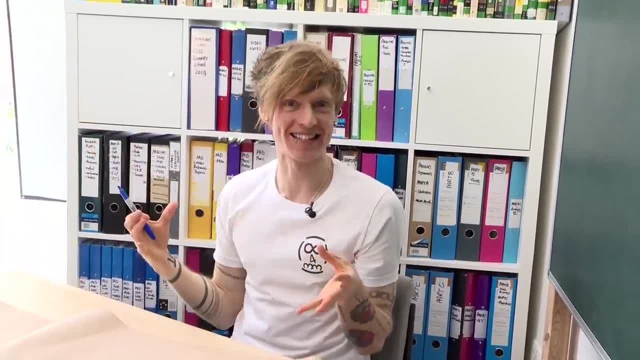 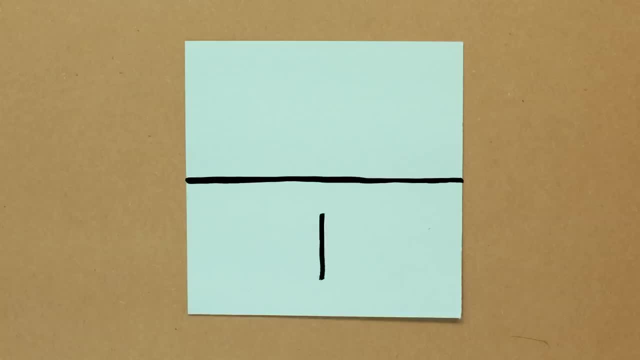 problem and see if we can use that to build other cases. If we start with the two that we had, we had a square and we divided it into two. So if I now divide this bottom rectangle into two squares, I've now got a square that I can divide into two and another. 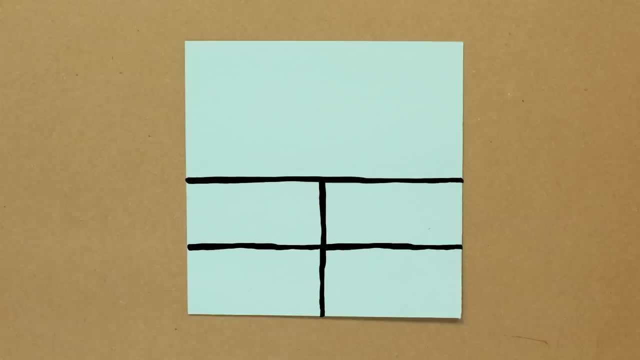 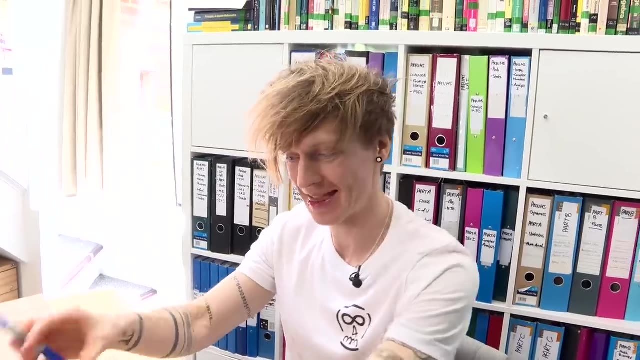 square that I can divide into two, and lo and behold, we've got a solution. So we've got five. there n equals, five is a tick, So we took what we had, which was two, and then sort of broke it down. 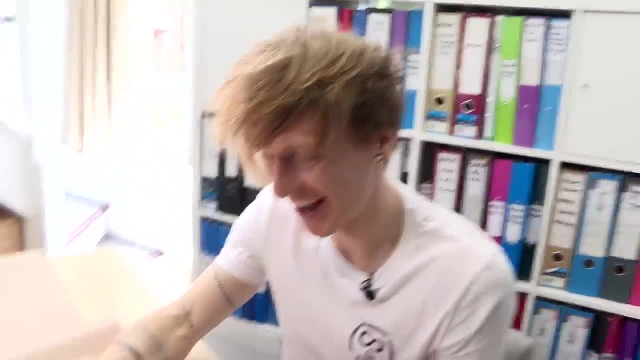 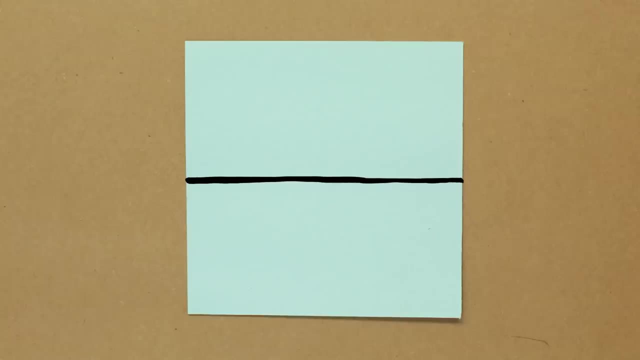 so I call this the breaking down method into one of them. We broke it up first into two, two squares, and then copied what we did at the start to get four. So we replaced one rectangle by four rectangles, so in total we added three to our two that we started with. Now there's 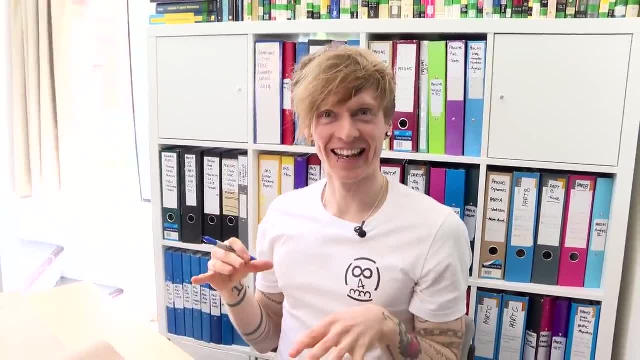 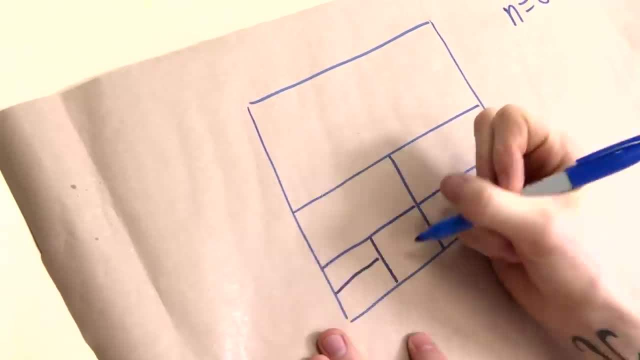 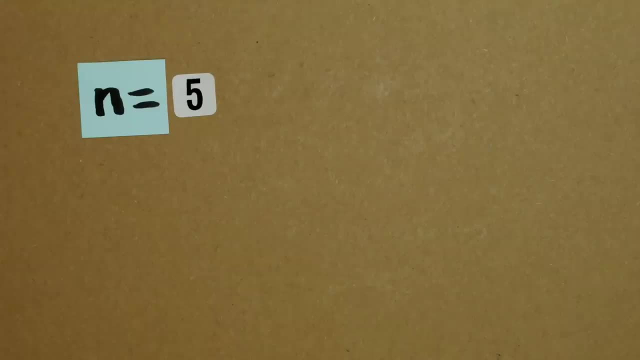 nothing stopping me from doing this again, and again, and again. So I can pick one of my five rectangles, divide it into two squares, and then divide each square into two rectangles, And now I should have eight. One, two, three, four, five, six, seven, eight. So now we get n equals. 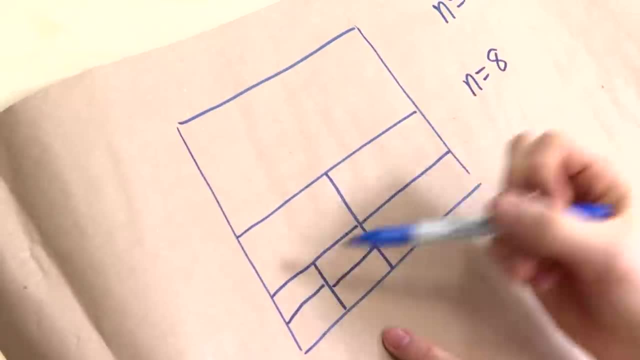 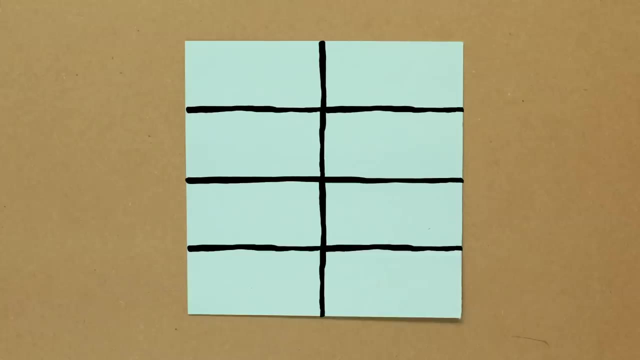 eight is a solution, And I could have, of course, picked another rectangle and divided that up. I could have picked the top one and then I would have got a solution where we had eight all of the same size. But remember, we're not interested in the specific configuration, We just care about. 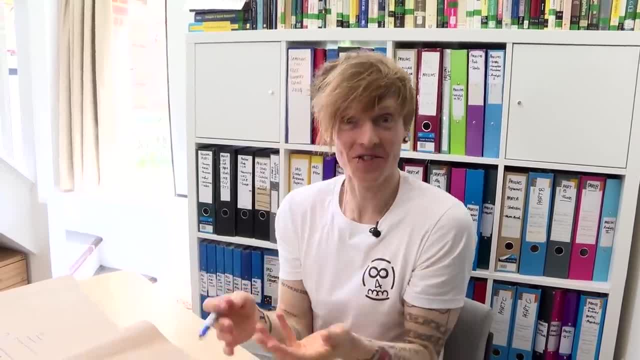 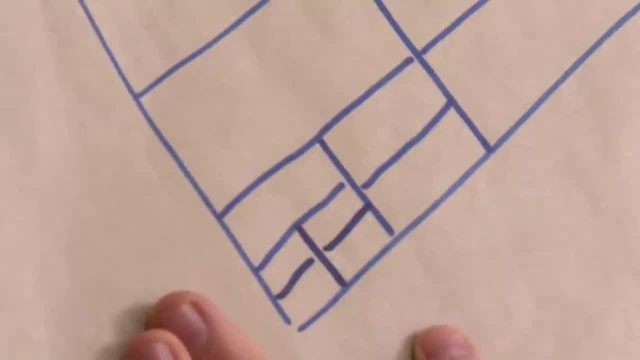 the number of rectangles. Is it a tick or is it a cross? I can continue to do the same thing. So, if I continue with this bottom left, one, two squares, two rectangles, And I've added, I've replaced one rectangle by four, so I've added three. 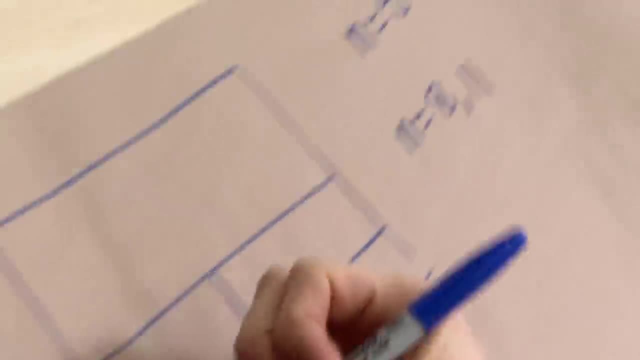 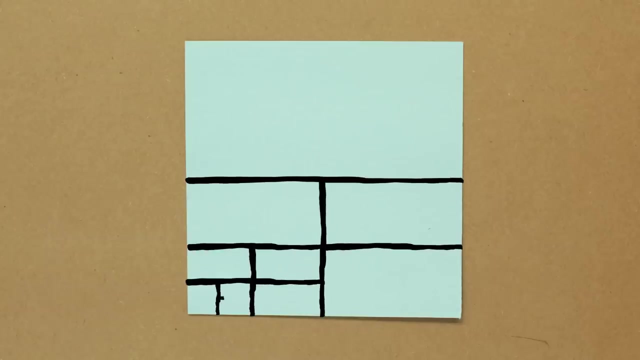 so that would be eleven, And I can do the same again. So there's the last one I'll show you, because I'm running out of space And I can just continue this. And again, I don't have to keep picking this one, We can keep adding three. So we get 14,, we get 17,, we get 20, 23.. To come back to 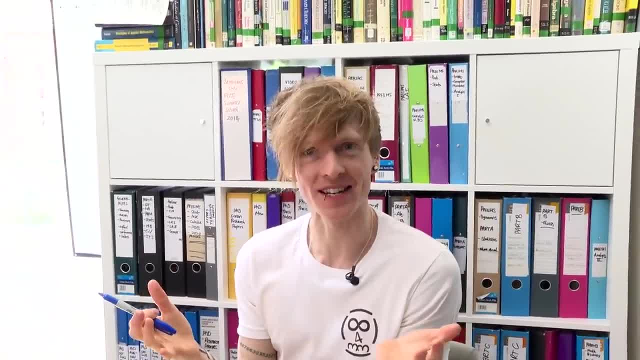 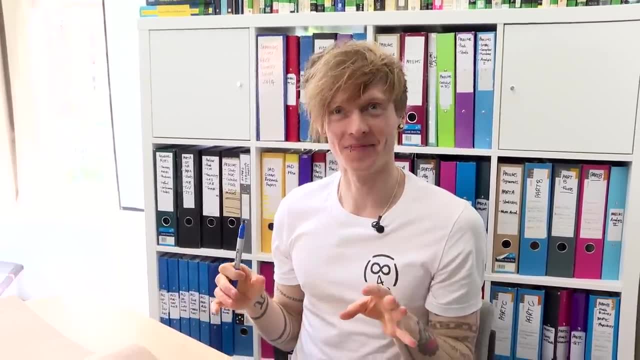 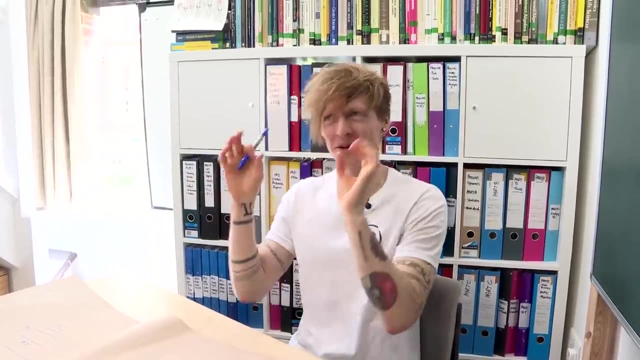 the original question for which: how many like ways can we do this? We now have an infinite number of ways to fill a square with these two by one rectangles, Because we just keep adding three and we can just go on forever, But we're missing quite a few. There's a lot of gaps. There's almost like twice as many gaps. 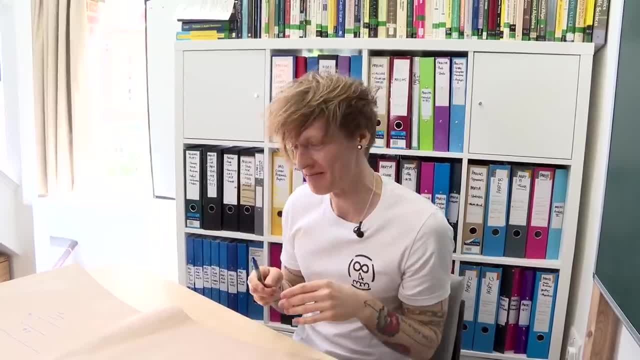 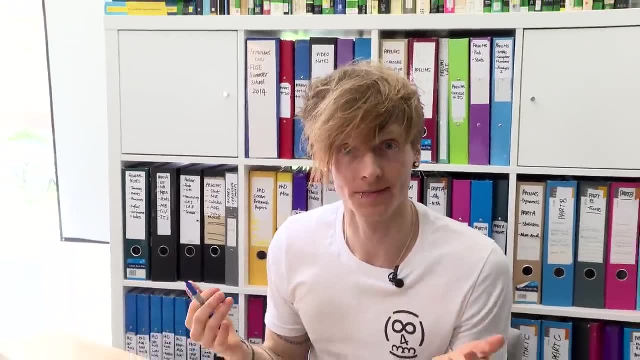 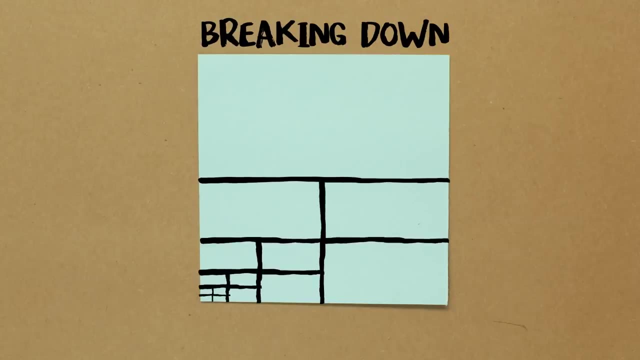 as there are numbers we're hitting, because we're hitting every other third number. So what we want to try and do now is think about: well, how could we hit those numbers? This method I called the the breaking down method, because we took a solution that we had and then we broke down a rectangle and added three to the total, And then the other. 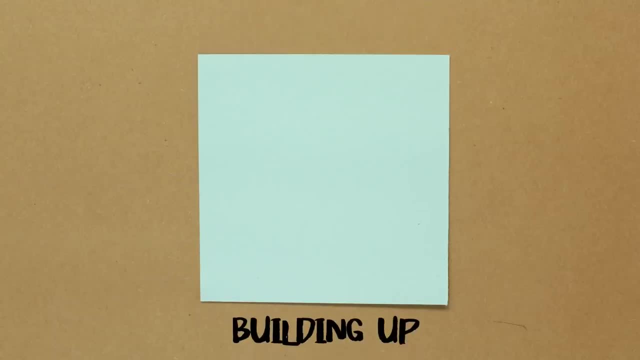 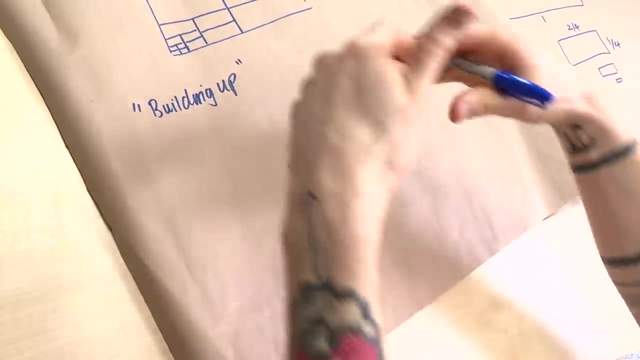 approach. I'm calling the building up, Because what we're going to do is again start. we're going to start with our square and we want to now add rectangles around the outside, But so that the final shape is a square, Because, remember, the square can be any size. So if we try and build, 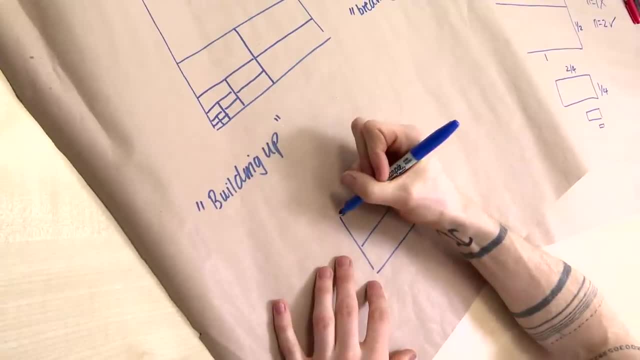 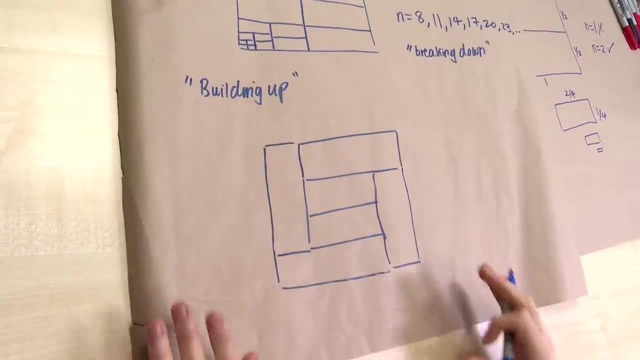 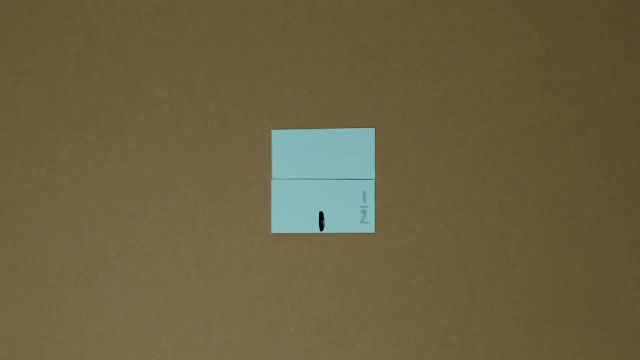 up, you think about this a little bit and again, you should do this. You can kind of create an overhang like this on all four sides. You can hopefully see that's possibly going to work. It could maybe be a square. So again, if we take the middle one to be one and this one to be a half, 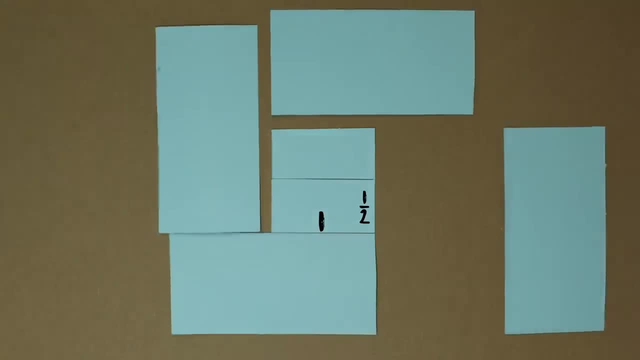 So the middle square was one by one. Then what we've got is: we've got a square and we've got a rectangle. So what we've got here is this length is two, And then this one, to be in the correct ratio, has to be one. So we do indeed have a square. We've got two different sizes of rectangle. 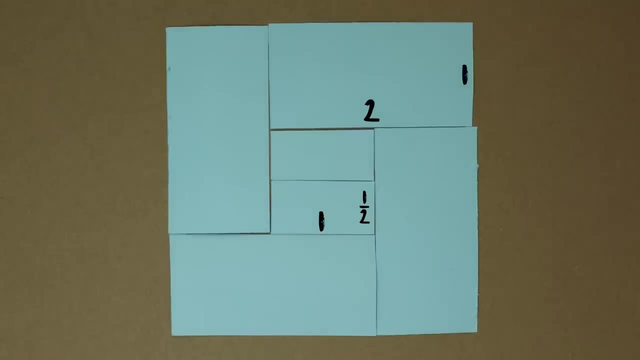 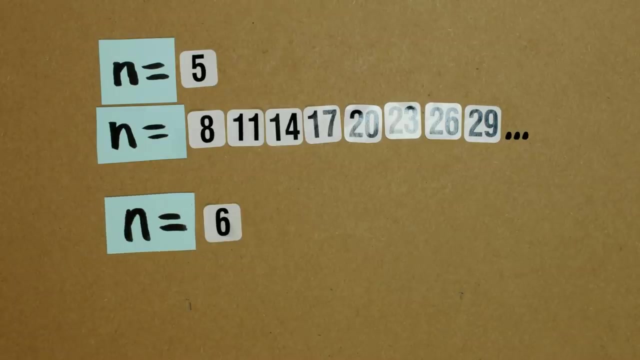 Two in the middle and then four of this second size, where the square that we fill in total is going to be three squared, But it's built up of six rectangles. So now we've got a different solution: Six We didn't have before And, just like before, we can keep doing this and building. 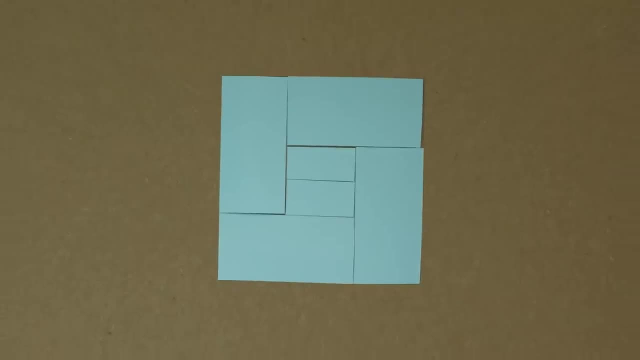 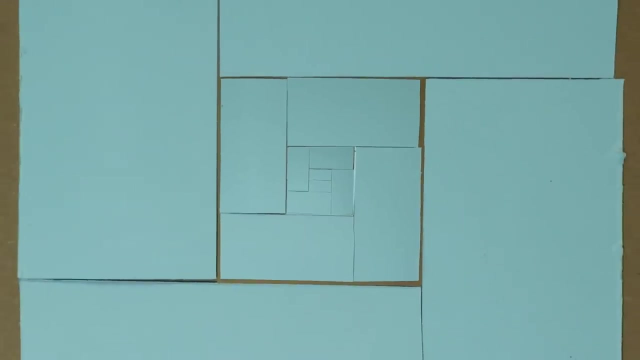 up So you could just do that And you could figure out the numbers. These are going to be a bigger again And you're going to keep doing this And we keep adding four every time. So we've got six, Then we can say that we can do this now for 10.. And we add another four to get 14,. 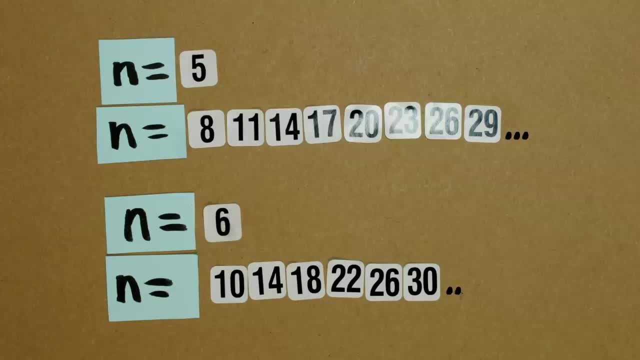 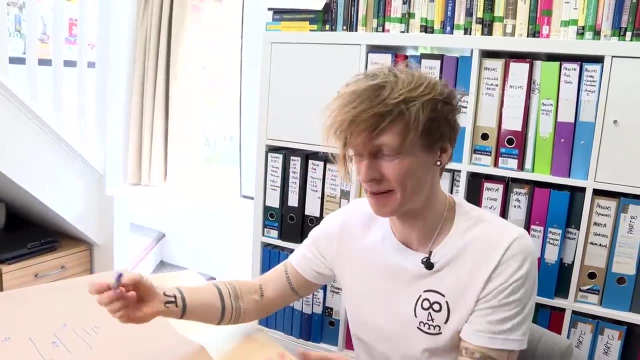 18,, 22,, 26,, 30. So we have another infinite list of possible solutions, And some of these numbers are the same. We've got 14 in both lists, But also, you know, we've got 10, which we didn't have. 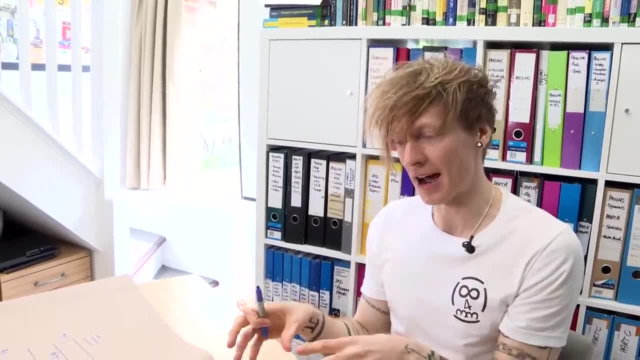 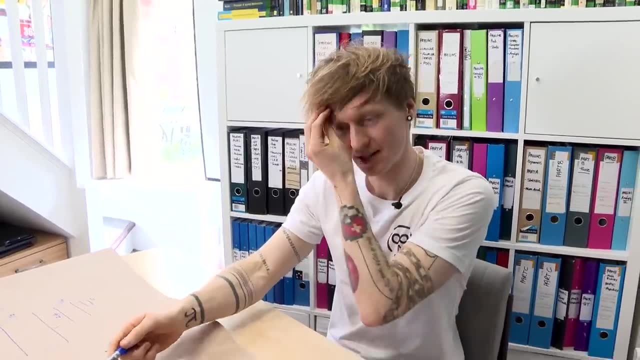 We've got 18, 22.. We've got new numbers as well, So there's some overlap, But we've got another way of constructing these solutions, Like before. in this first case, we said that what we were doing was we were adding three every step. 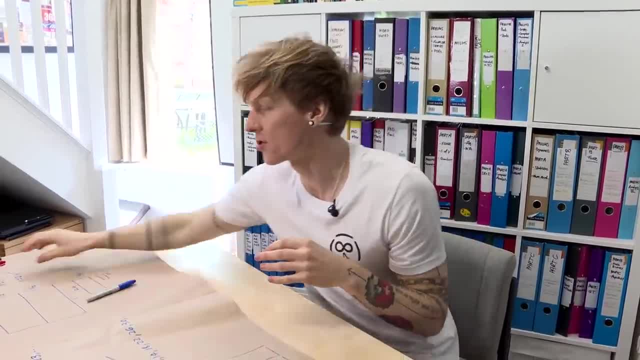 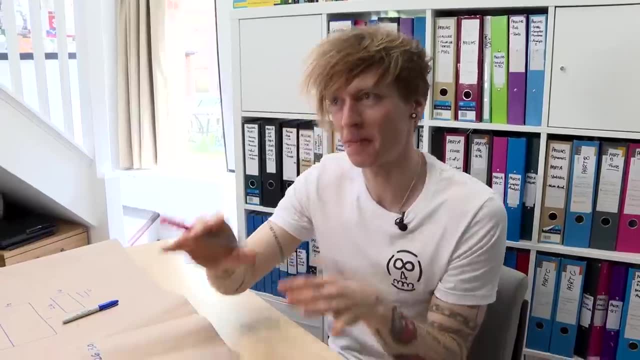 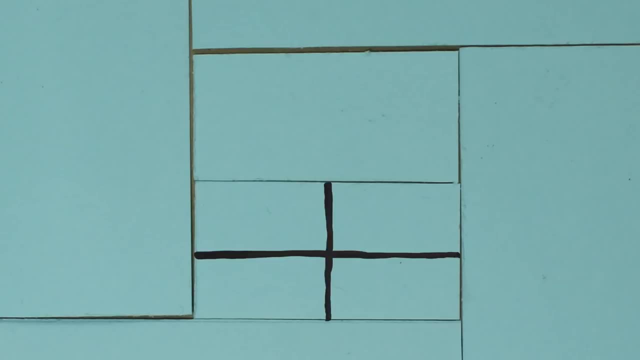 And you can think of this as saying: well, if I have a solution for n, for some number, then I know from our method here, the breaking down method. I can take one of the rectangles in the solution, divide it up into four smaller rectangles And that added three to our solution. 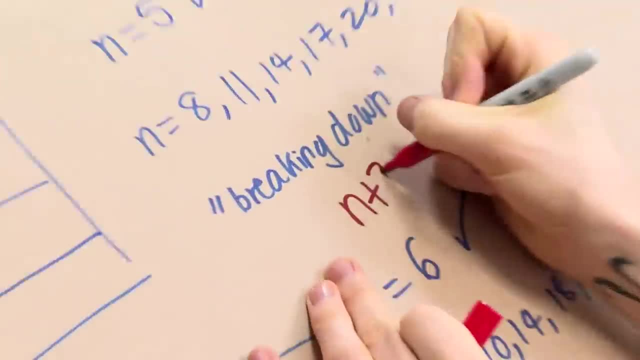 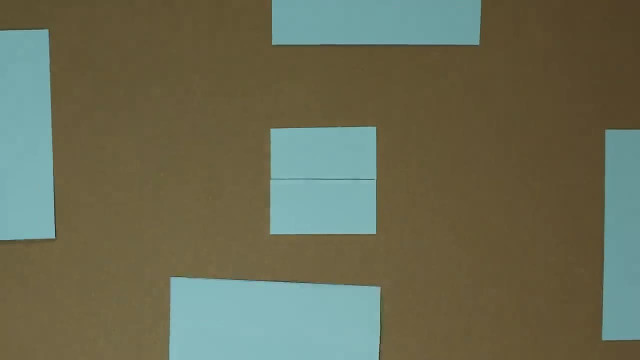 So if we had a solution for n, we can always get n plus three from the breaking down method. And then here we've seen the same thing, Because we started with two and I added four around the edge. But if I started with the five solution here, then I add four around the edge And then 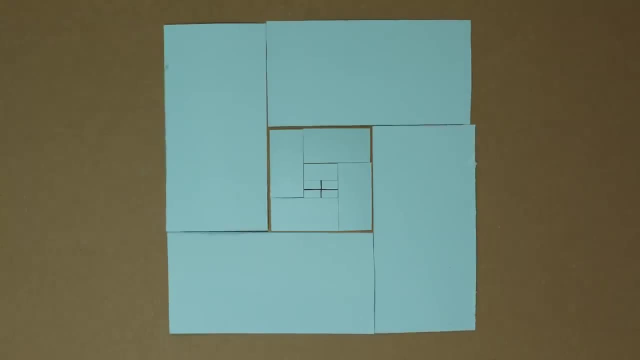 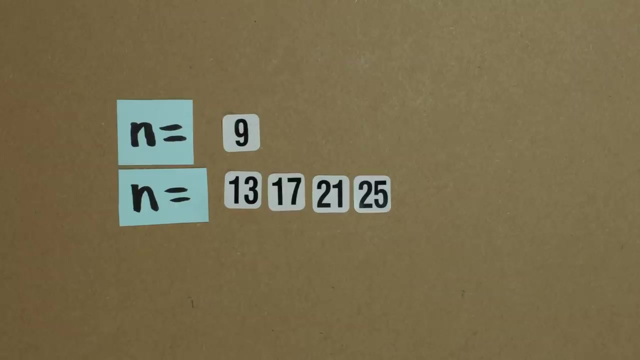 I add another four, So I can also get, for example: there I would get n equals nine plus four on that, So then I'd get 13,, 17,, 21,, etc. And again we're getting some numbers we didn't have. 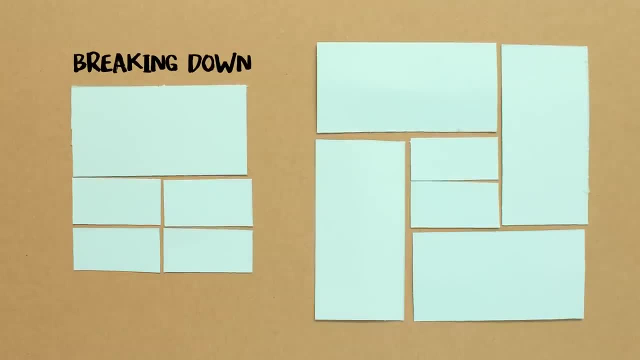 The breaking down method. if we can do it for n, we always get n plus three. Break one of them into four pieces: The building up method. if we can do it for n, we can always do it for n plus four. 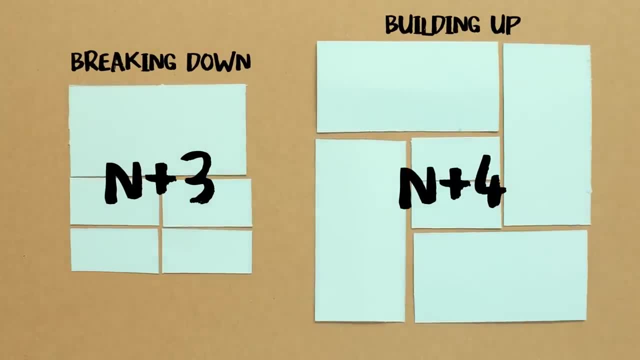 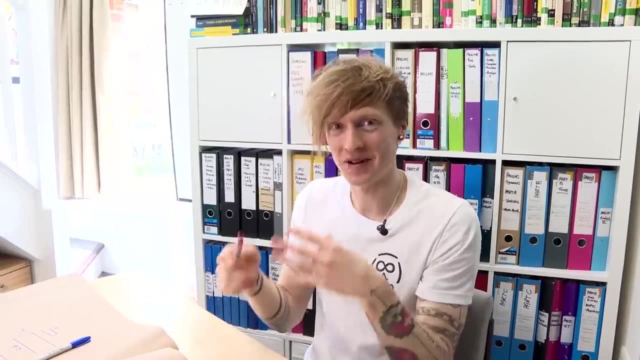 And now these two are really powerful rules. So we've already seen that we've got a lot of solutions. But if we actually think about this mathematically now using the algebra, we can begin to see that we actually get almost all of the numbers. 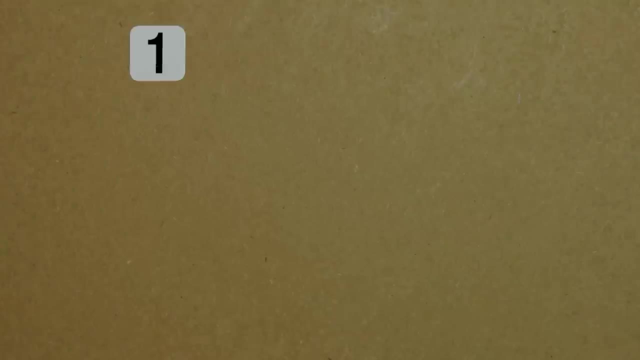 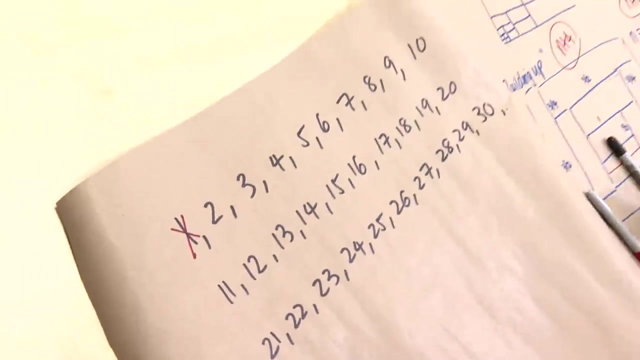 So I think the best way to demonstrate this is to sort of write out the list of the first numbers and cross off the ones we can and can't do, And then we'll think about: can we prove this So we know that one didn't work. I think that's the only one we know that doesn't work. 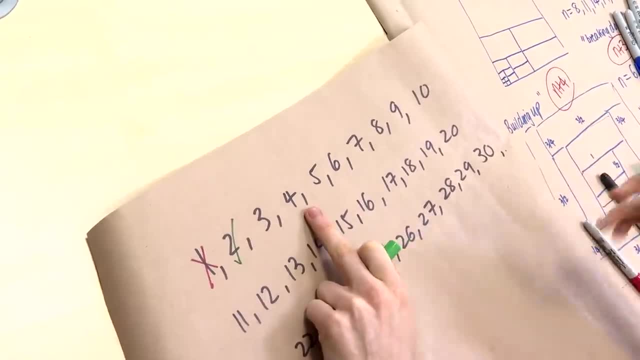 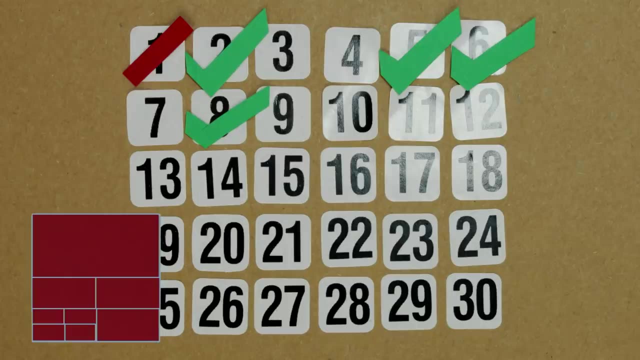 We showed that two did. We haven't looked at three or four. We had five, We had six. We haven't covered seven yet I think we had eight. Yes, eight was the five plus three, Nine. we got down here by doing five and then four around the outside. Then we had ten on our list. Now we've 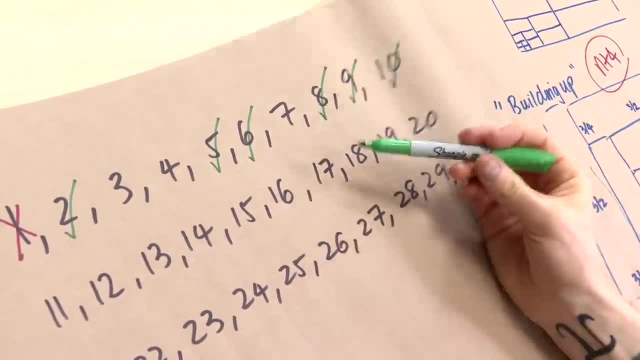 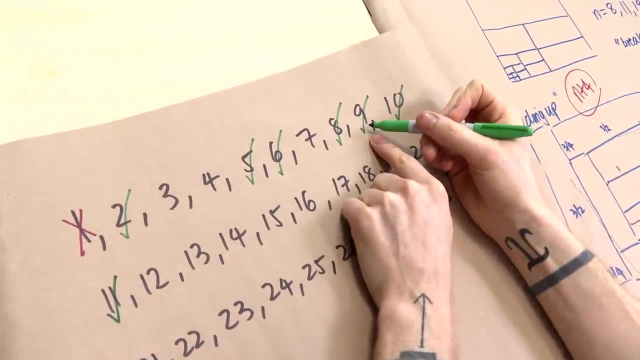 got something really helpful here, because we've got three numbers in a row. So because I've got eight, I know that I can just add three to it and get eleven. Because I've got nine, I can add three to it and get twelve. Because I've got ten, I can add three to it and get thirteen. And then this is. 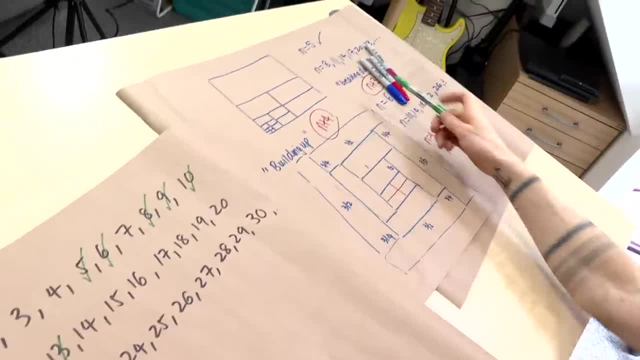 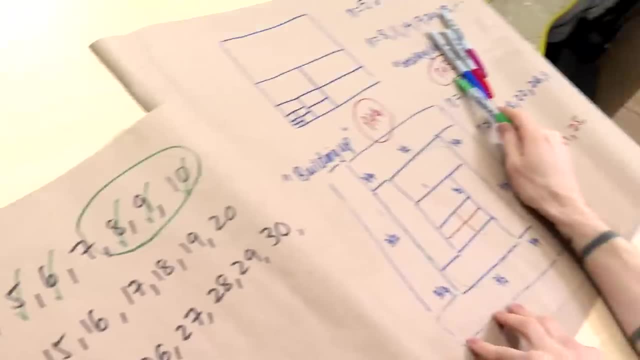 just going to carry on So you can look back through our lists as well and see, you know, we had fourteen, seventeen. You could tick them off, But if you spot that, because we had these three numbers in a row then and we had this n plus three rule, we're actually going to get. 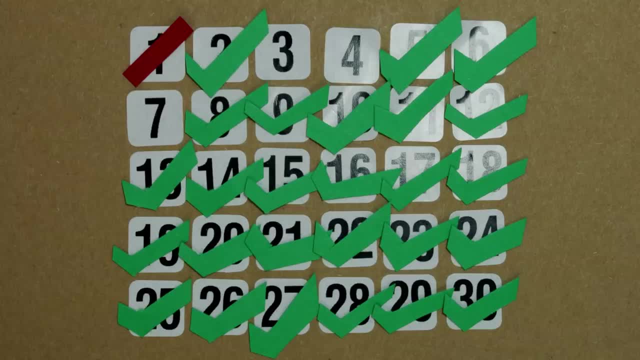 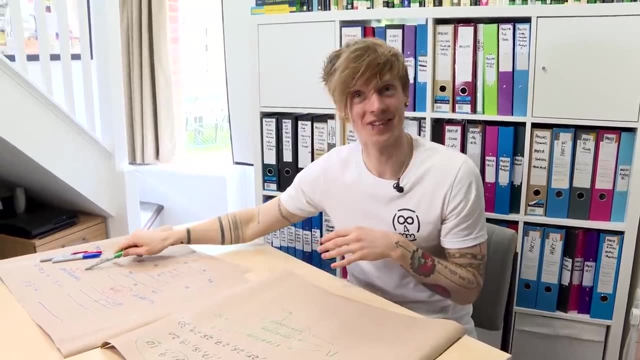 all of the other numbers. So there's lots of ways of spotting that you're going to get all the other numbers. But however you do it, it relied on the fact that we had- well, actually only really this rule, the n plus three, once we figured out that we could get eight, nine and ten. So we did need 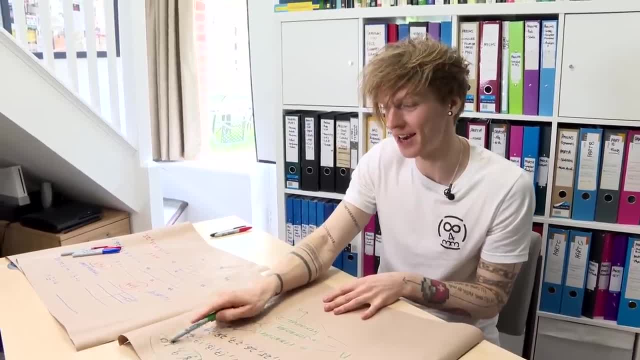 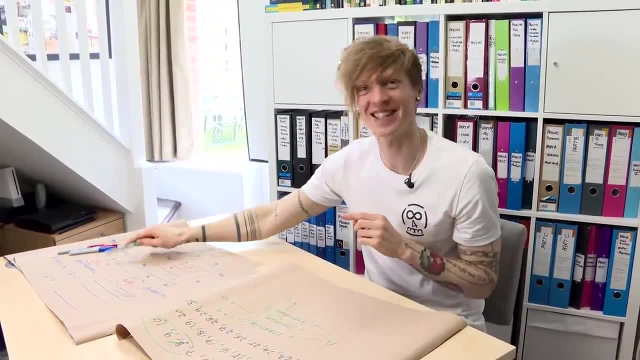 building up to get some of these right. So nine and ten came from the building up method and eight came from the breaking down. So we did need the second method, but really we just needed the n plus three rule plus those three and then we got all of the numbers. So that just leaves us with. 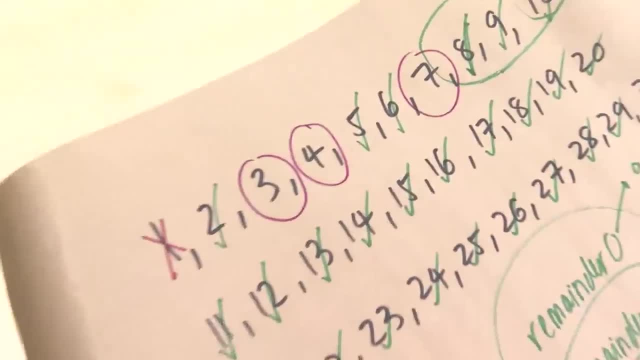 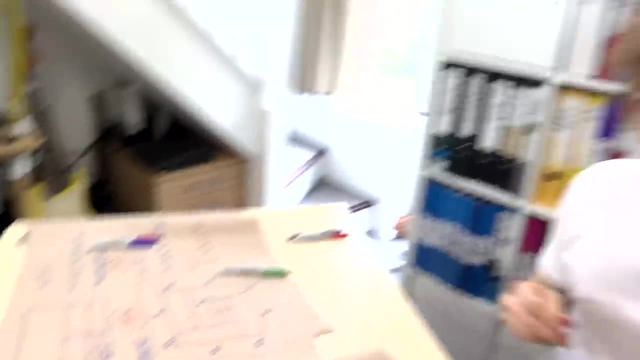 three, four and seven. So we know that one's impossible. We know that every single other number is possible now except three, four and seven. So we've got to figure these ones out, And this is: you've got to do this case by case. I'm going to need more paper, aren't I? 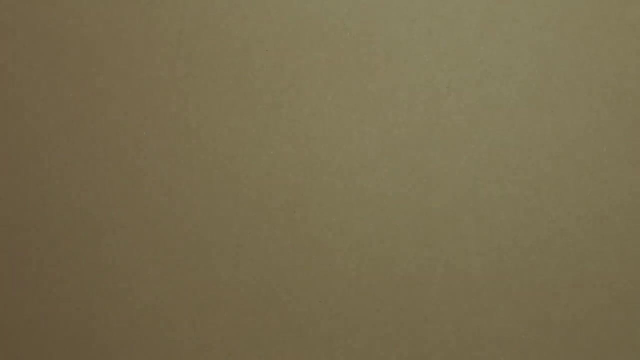 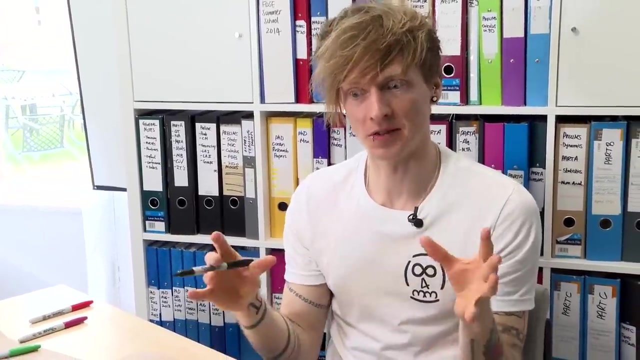 I have no intuition as to whether three, four or seven are possible. This is how I think about it. We're going to consider three. We're going to say, right, let's try and find a solution for three, Suppose we can do that And you want to think. 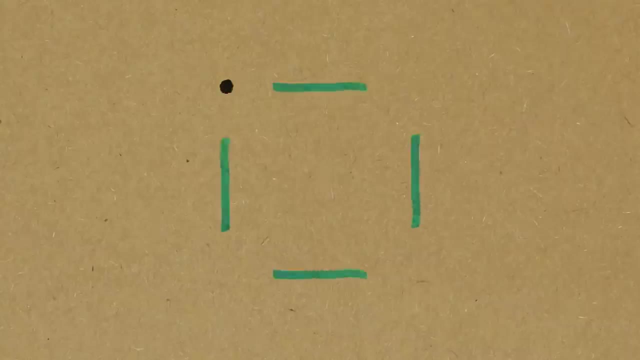 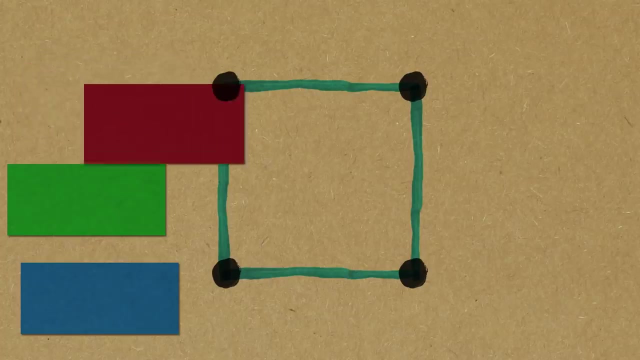 about the number of corners in your square: One, two, three, four corners And we have three rectangles, For example. let's take one of our rectangles. Suppose it hits all four corners. It's clearly got to be a square and there's clearly no space. 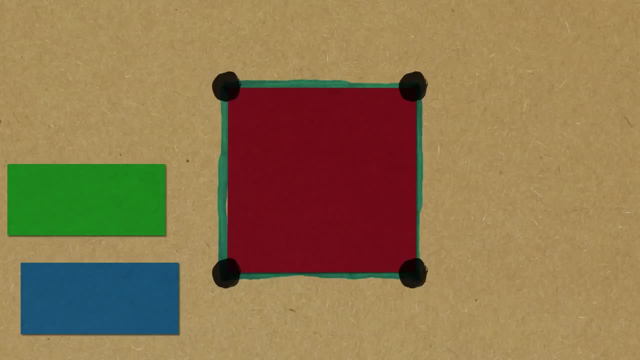 for the others. So you cannot have one of your rectangles hitting all four corners. Similarly, you cannot have one of your rectangles hitting three corners, because if one rectangle hits three corners it kind of has to hit the four and it kind of has to be a square again. 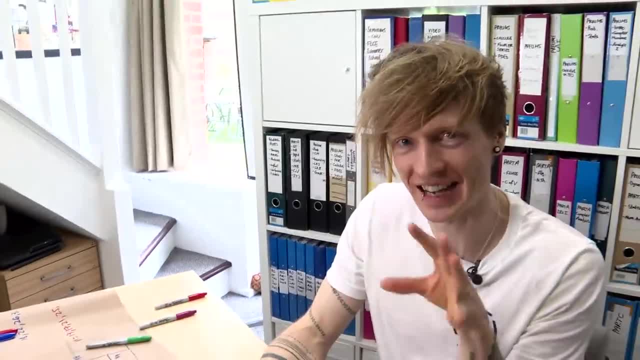 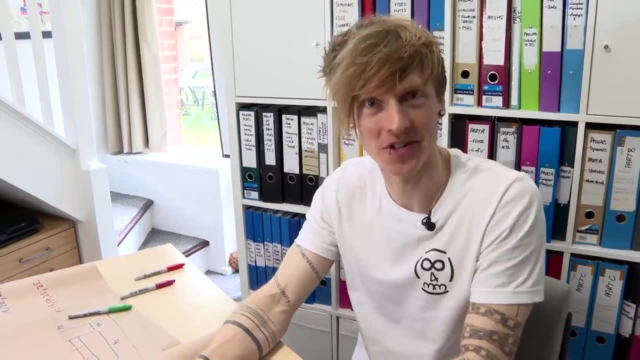 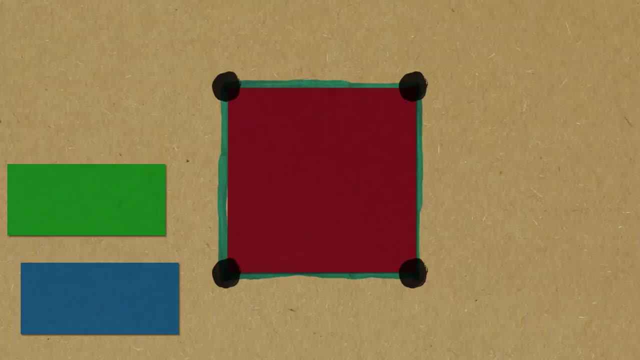 So the highest number of corners a single rectangle can hit is two And in fact one of them has to hit two because there's only three rectangles and four corners. So categorically we can say: one of the rectangles must cover two of the corners of our square. 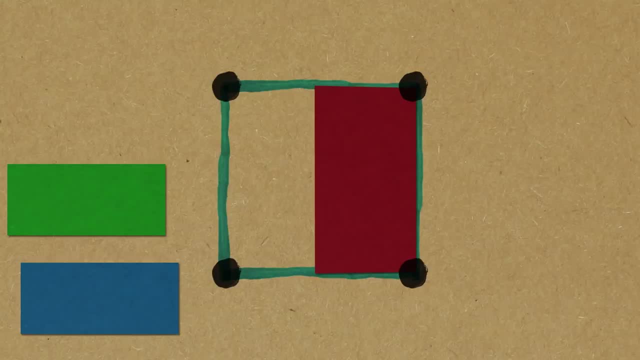 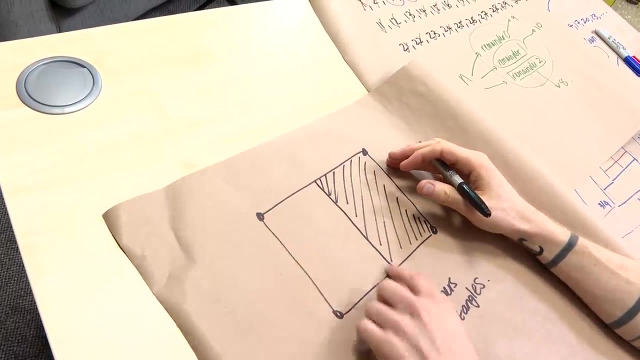 And so the only way to fit that is to divide it in half. If we're trying to find a solution for n equals three, this is completely fixed. There's nothing else that can happen. So then we've got to fill the remaining space. 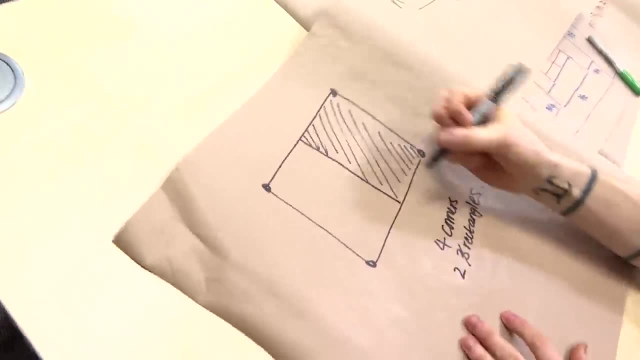 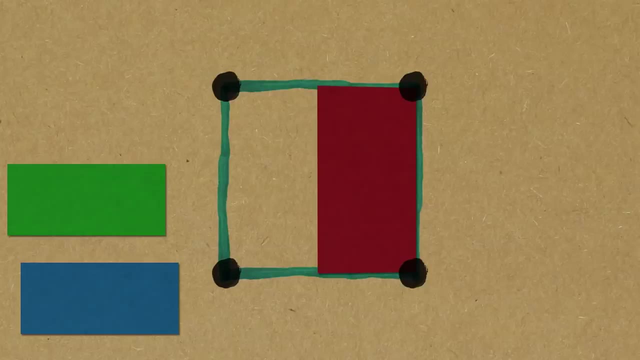 with two rectangles. So now we've got two rectangles and we've got four corners Again. So, OK, it's a rectangle instead of a square. but the corners is a really helpful way to get stuck into this problem, because they've all got to be touched. So now you say, right, I obviously can't. 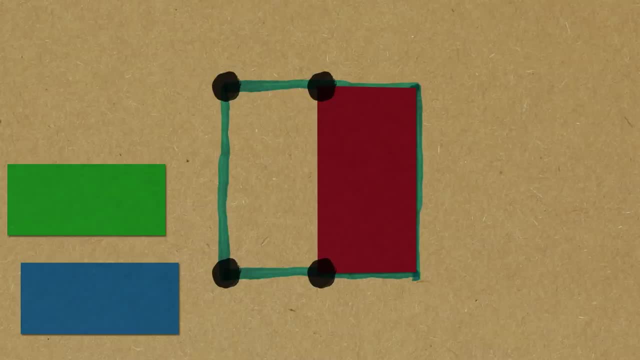 hit all four, because then I'd fill it, It would work. But I've got one rectangle left. I can't hit three for the same reason, So I have to hit two, and each of them has to hit two. If you take a one by one square, this is a half, So this one has to be a quarter. It's the only way you can. 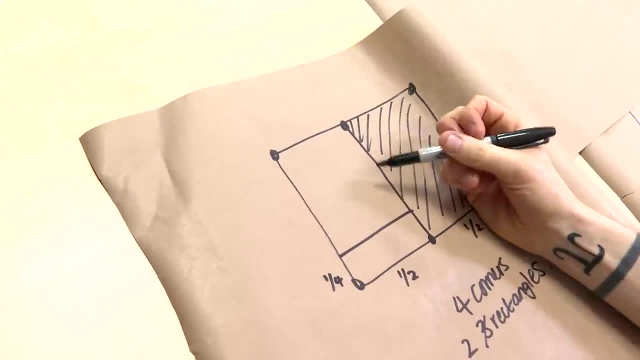 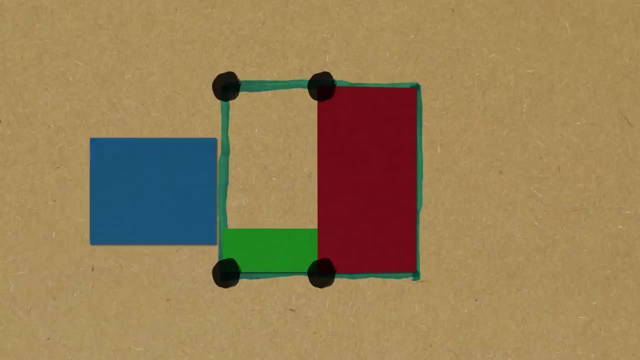 fill a rectangle fitting two corners. So then what we're left with this has to be a rectangle, And if we figure it out, this is three quarters. This is a half. It's certainly a rectangle, but it's not in our ratio one to two. So that doesn't work, And so n equals three. 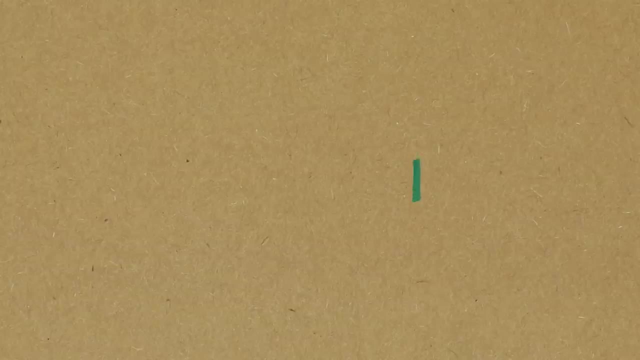 doesn't work. Three is getting crossed out, Now four. you do in basically the same way. Start with your square. You say you've got four corners. We can't. We've got four rectangles. Similar argument: One of them has to touch two, because if each one touches one, 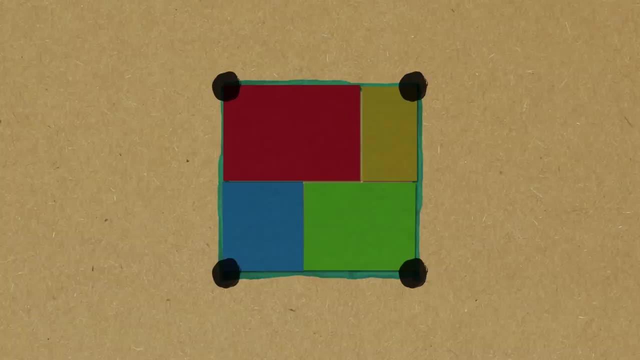 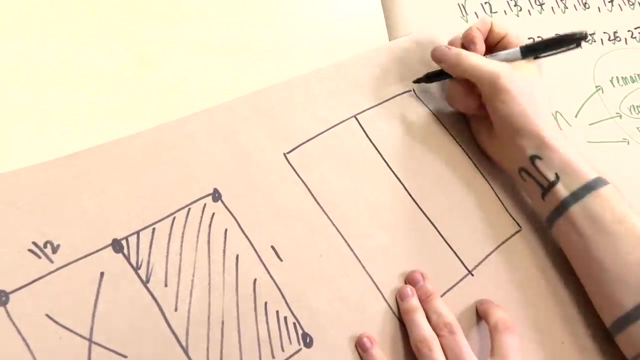 you can play around with it a bit, but you'll see that it doesn't work. It kind of has to be four, But the only way you can get it to work and it doesn't doesn't fit our rules. So again you have to have one of them like this, touching those two corners. So this is out, And then you're. 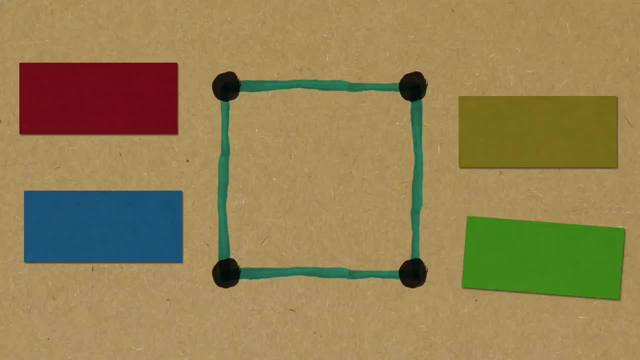 left. now with three rectangles to fill this half. We've got four corners, three rectangles. Same argument as before, except now we're on a rectangle, We have to touch two, So it has to be this one half by a quarter again, And then we've got the same space You can play around. 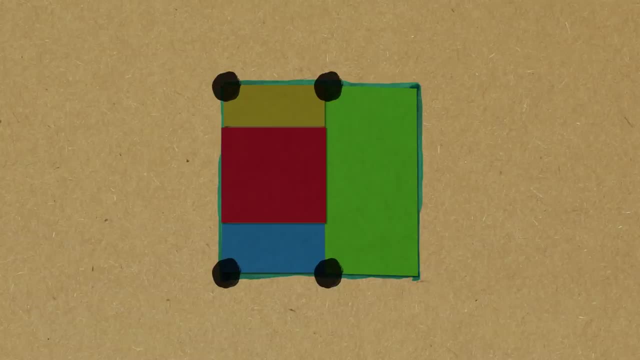 with this as much as you want. If you put one horizontally, it has to go the same size- a half and a quarter, And that's obviously a square. Or if you go vertically down, this won't work, because this is a quarter and this one here is three quarters. 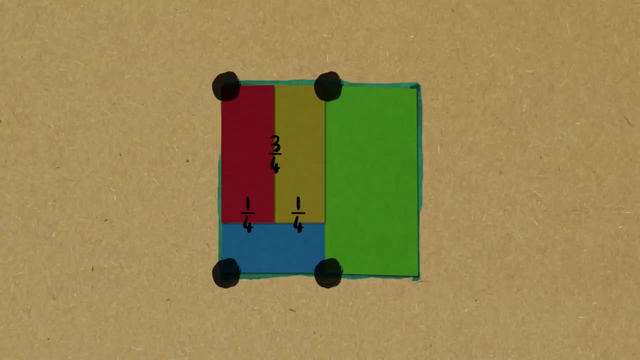 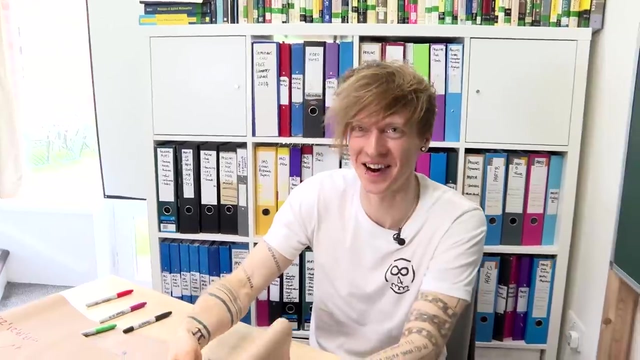 That would be one to three ratio, not one to two. So four. for the same reason really, as three ain't going to work, Cross it off, So it all comes down to seven. This is the big finale of our infinite list of numbers for solving my favourite rectangle puzzle. Can we do it? 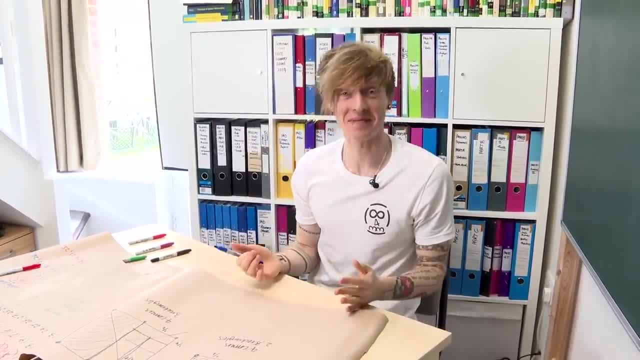 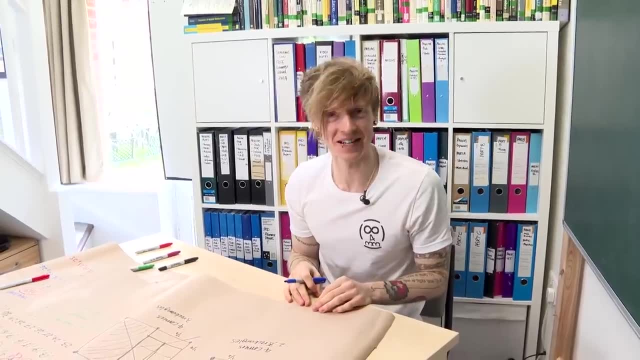 for n equals seven, And the answer- maybe surprisingly- is yes, we can do it. It is possible for seven. It's quite tricky. For those of you who really want to give this a go, this is the time. Have a go. It's very fun trying to do this. 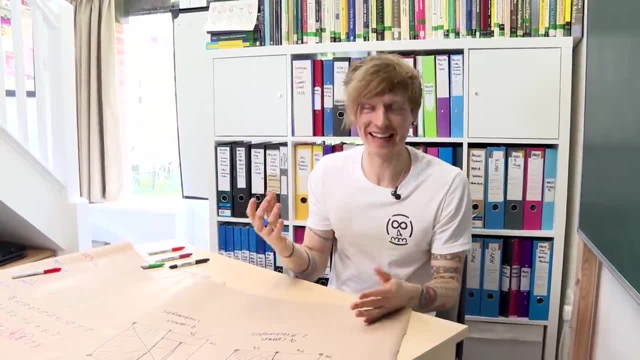 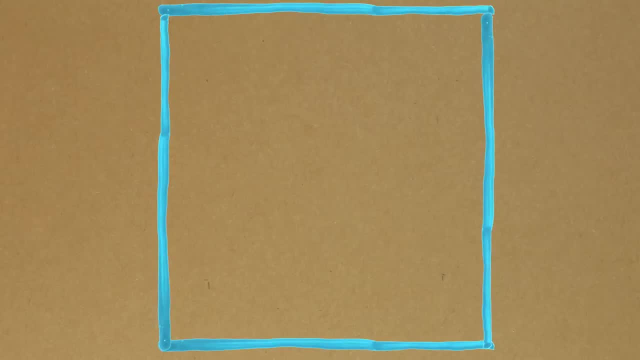 The trick with solving it for seven, or the way we do it, is we actually need three different size rectangles. We'll say this is a one by one square, so I can convince you all that this works, and it doesn't look like it's going to work at first. So to start with, we have one. 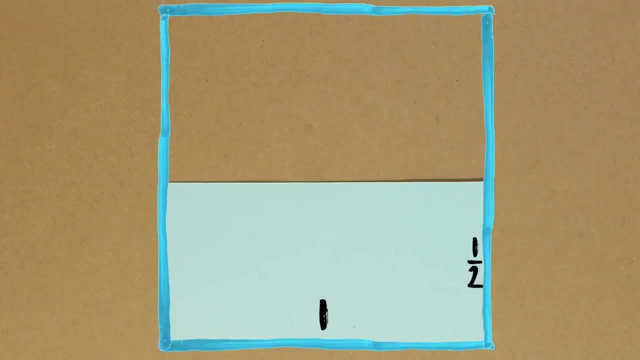 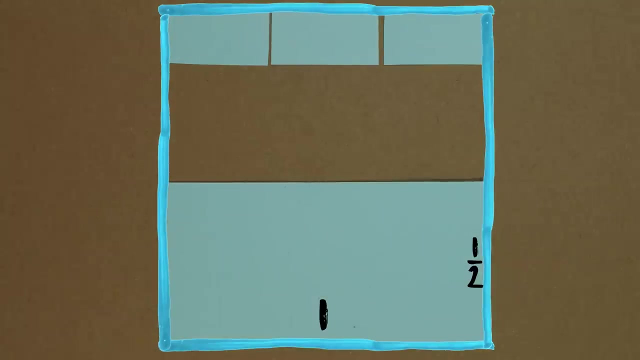 big rectangle that's going to be our half by one. So, you'll notice, this is the building block of almost all of our ideas actually. And then you have three little guys, So this is going to have to be a third for each of them. 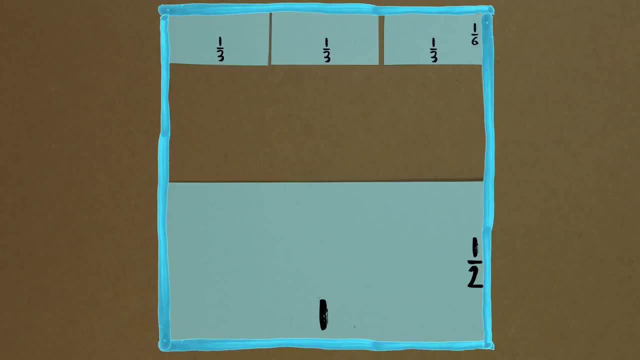 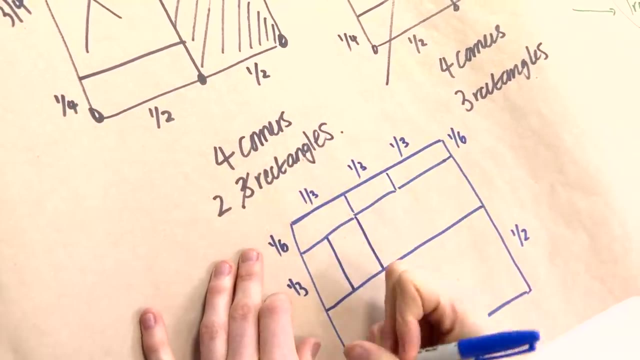 and the height here to be in the ratio one to two is one sixth. We have another one here and then we put another two here. This is a third, that will be one sixth and that will be a half, So we can check. one sixth, that will be two sixths, three sixths, So that's one That works. 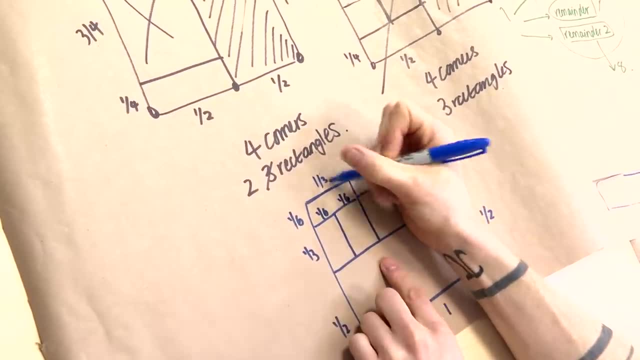 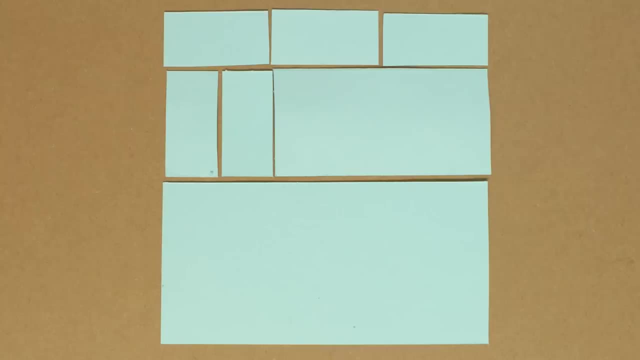 This bit here is one sixth, This one's one sixth, That fits to be one third. And then this gap here, this top long side, is two thirds, and this one's one third, And we're done. So we've got five of these small ones. 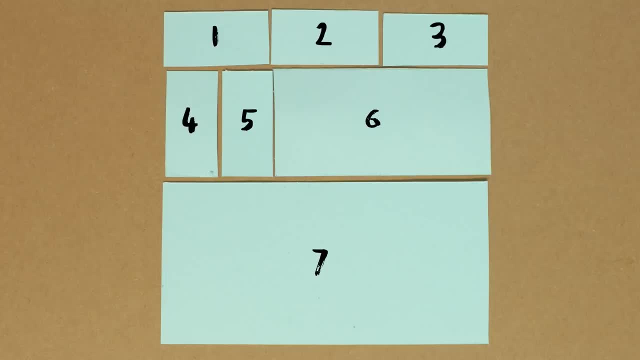 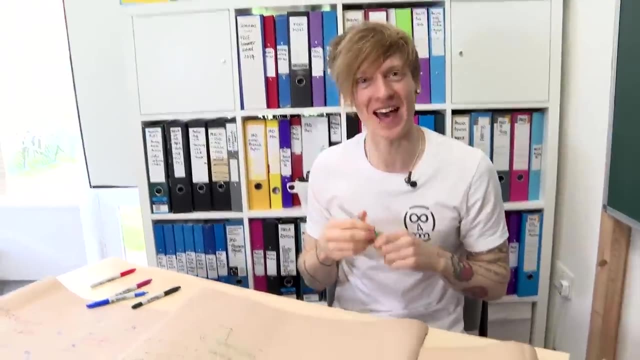 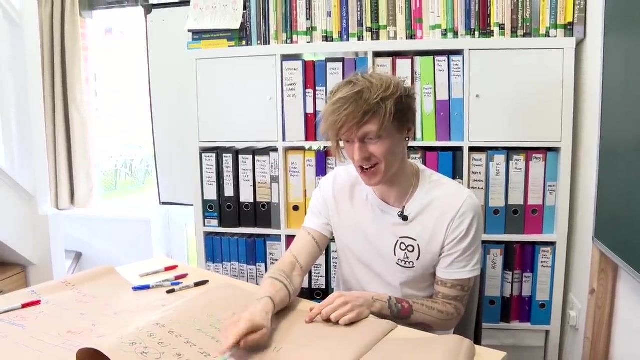 one middle sized one and one big one, And that is the solution for n equals seven, n equals seven, So we can solve it for all possible values of n. We can fill our square with n rectangles in this ratio two to one, except for one, three and four. 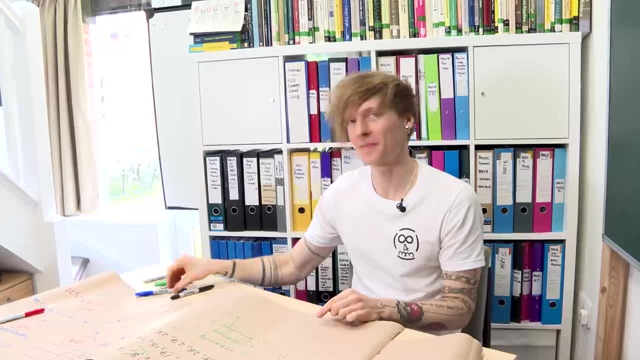 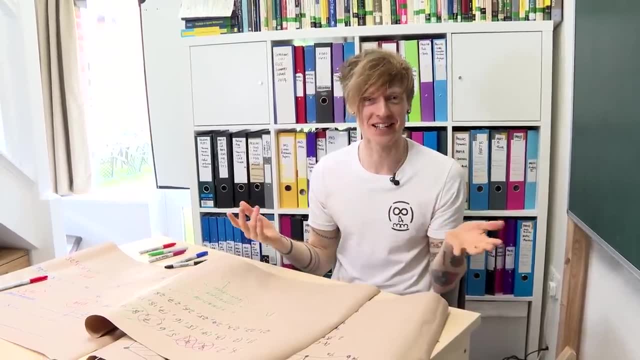 All right, So now anyone who watched this video can get into Oxford. Yes, I used this question for the last two years actually, So that's why I've had to retire it, because I tried to come up with new questions, but I like this one so much that actually this: 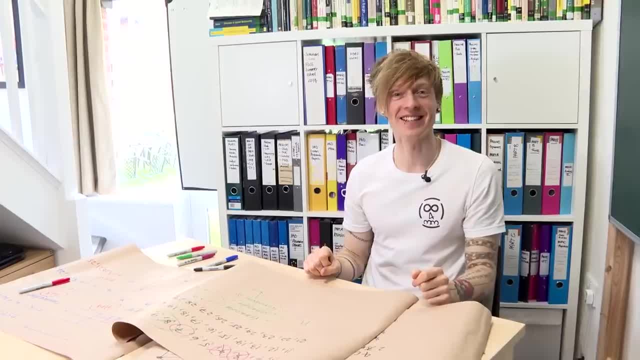 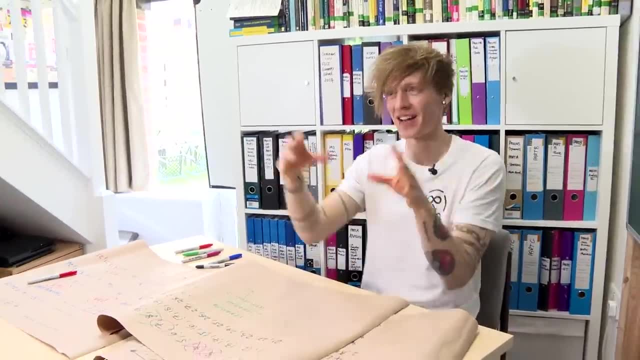 is the only question I've used on repeat, but it's now been retired. But yeah, this is the kind of thing, because there's lots going on, There's lots to think about, lots of things to check, and you could, if you wanted, go as fancy as you want in your proof with mod, arithmetic or spotting. 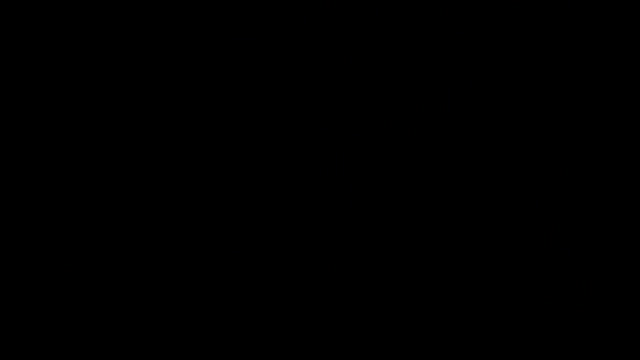 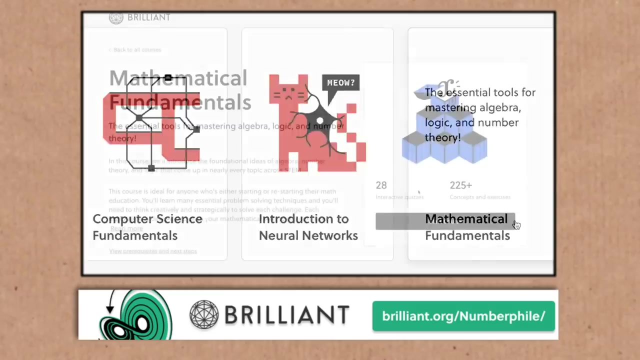 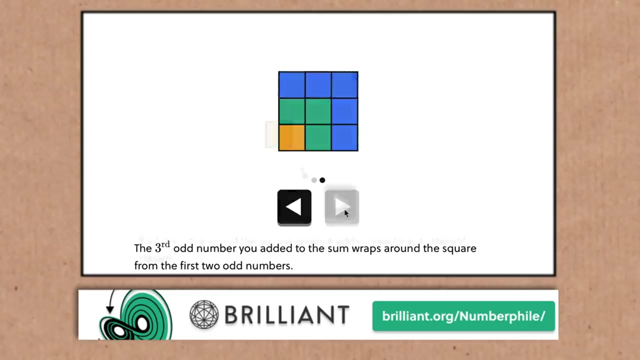 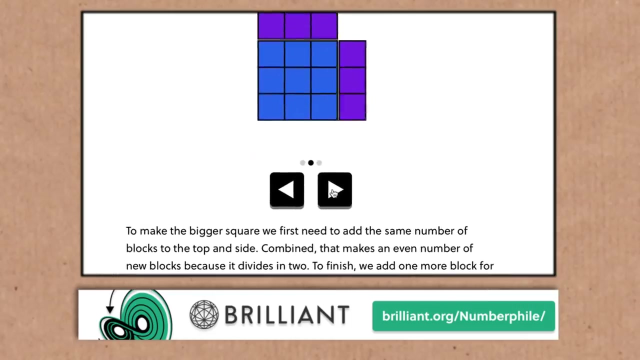 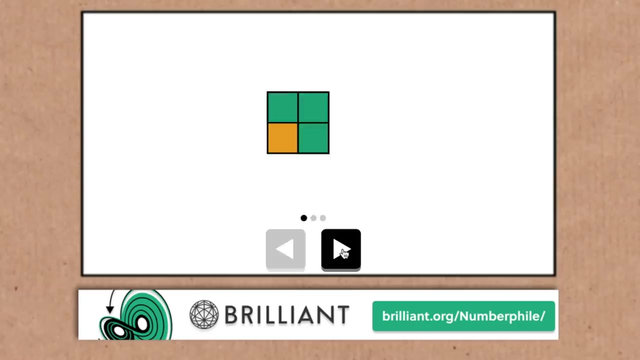 the pattern, But I don't think it's going to work. It's going to be a lot of work, So I'm going to go with this one. There's a lot to get stuck into. That's what the interactivity is all about. I never really think of Brilliant as being like 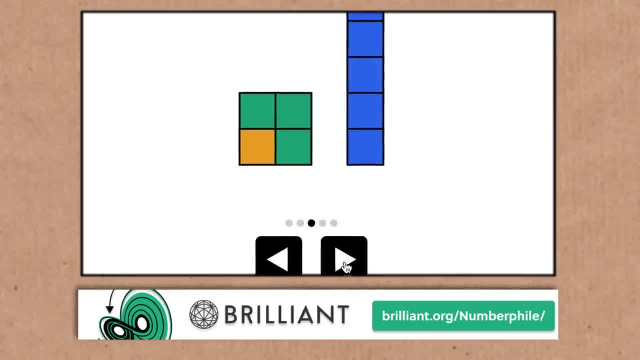 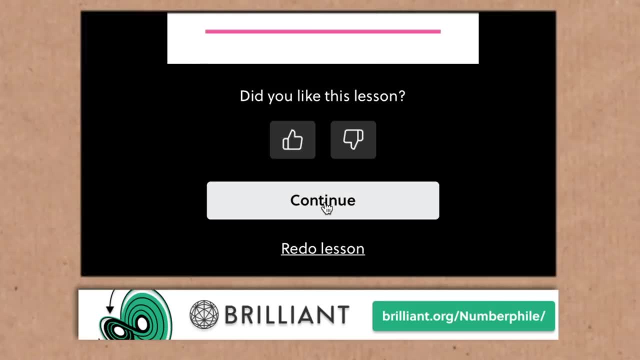 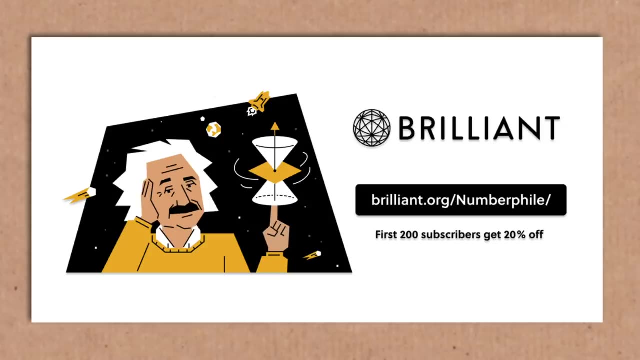 school or study. It's more like a series of fun puzzles, but each puzzle is secretly giving you a deeper understanding of mathematics or science. To check this stuff out yourself, go to brilliantorg slash numberphile. Using that slash, numberphile will tell them you came from.